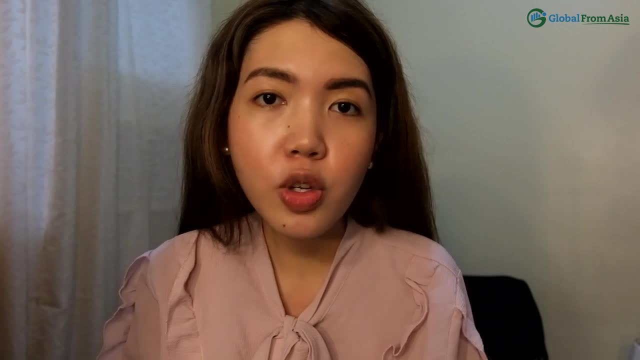 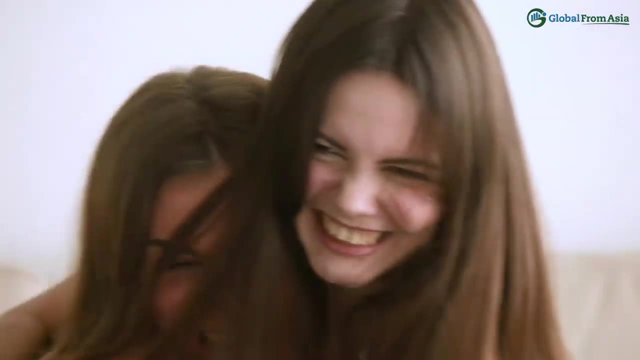 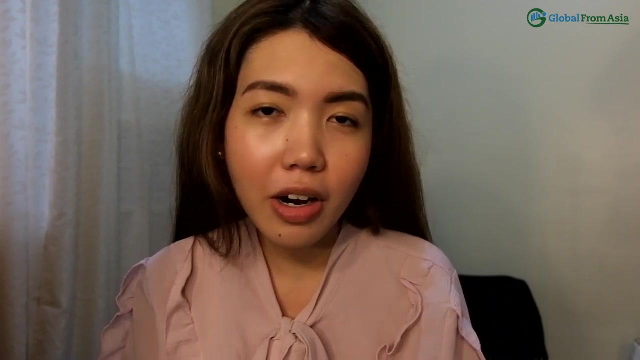 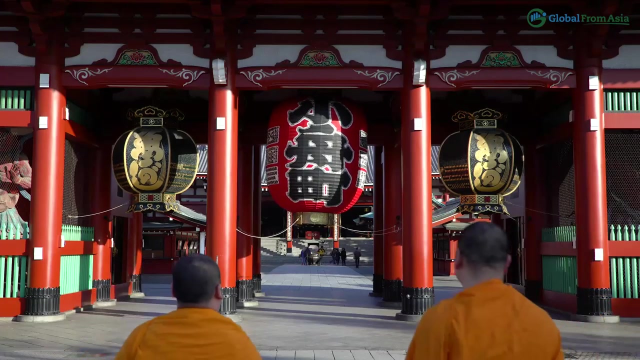 for them. Unlike in the western world, they can openly express their thoughts or feelings, because they are more liberal and practical in most ways. So let us discuss in this part the key differences in terms of different aspects. So in terms of religion for the easterners. 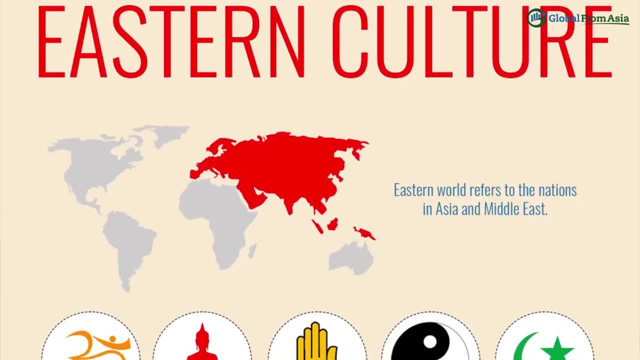 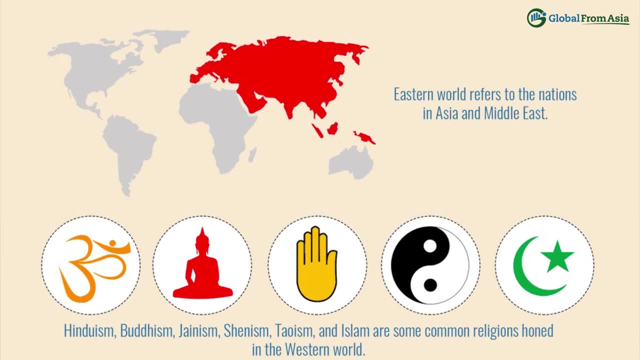 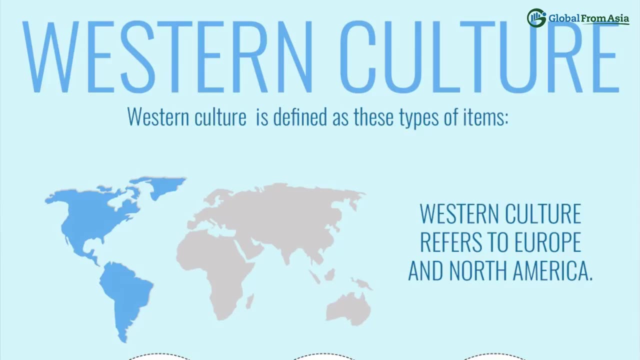 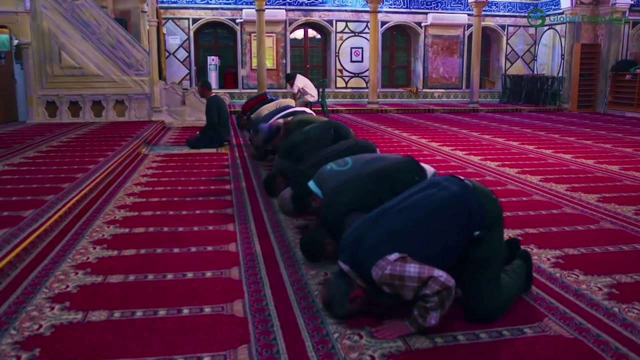 the most common religions there are Hinduism, Buddhism, Shintoism, Jainism, Taoism and Islam, While for the western world, the most common religions are Christianity, Islam and Judaism. Those are the three things that are the most common in terms of religion. 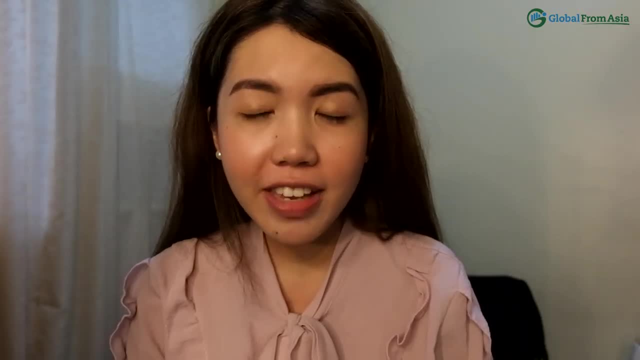 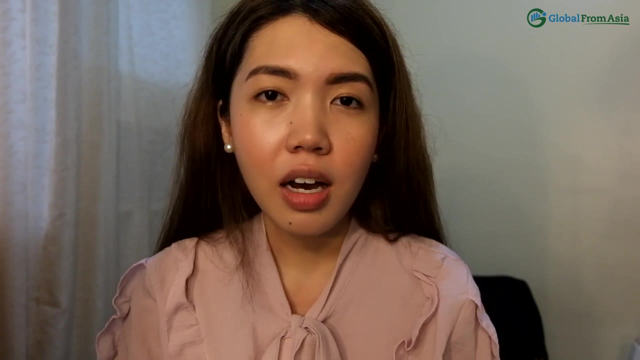 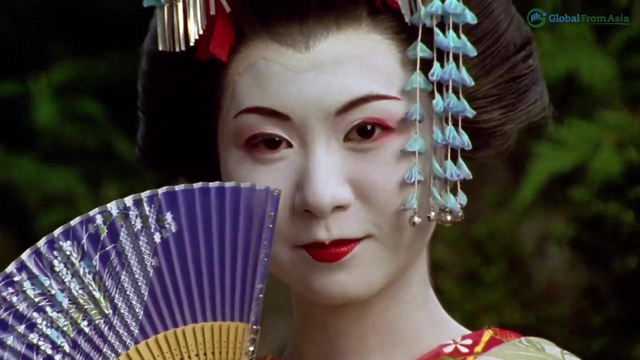 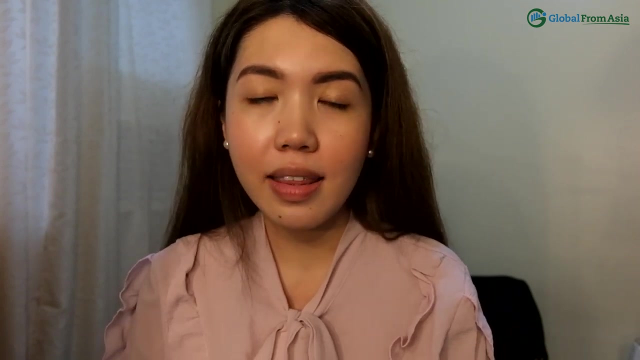 for the western world. So when it comes to expressing feelings, the easterners are more conservative, So they tend to cover their feelings because of fact and good manners and most of them do not want to hurt other people when they express their feelings, especially anger. But for the westerners, they are more open to express. 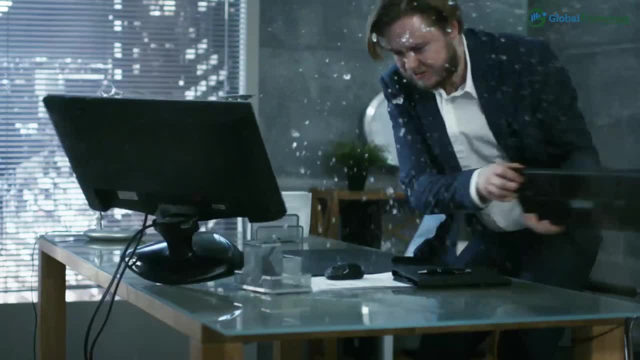 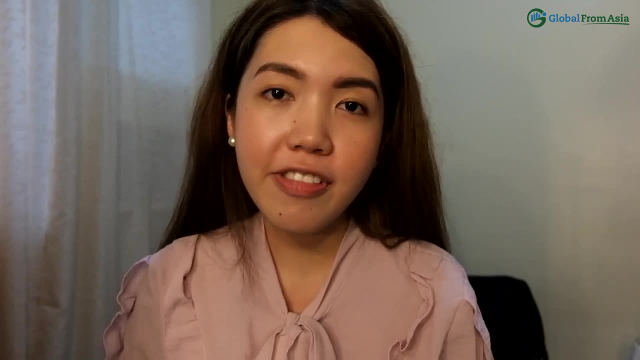 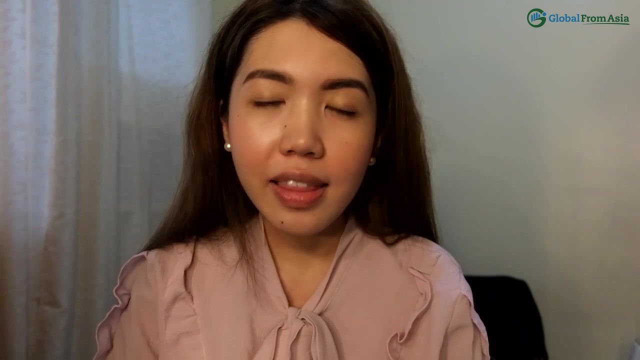 their feelings, so when they, whenever they are angry or whenever they are overjoyed, they actually express more and show what they truly feel, or what they truly think In terms of family and decision-making. religion delle: For the Easterners, the elders are actually the leaders of the family. 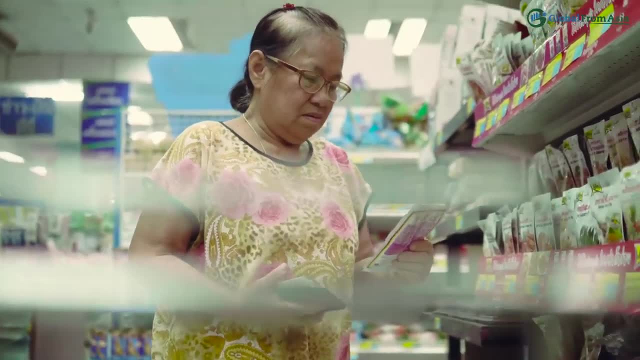 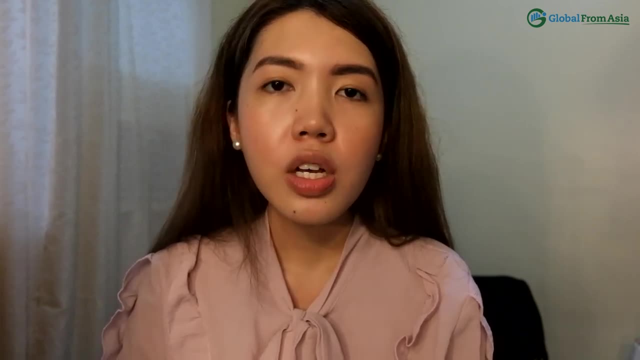 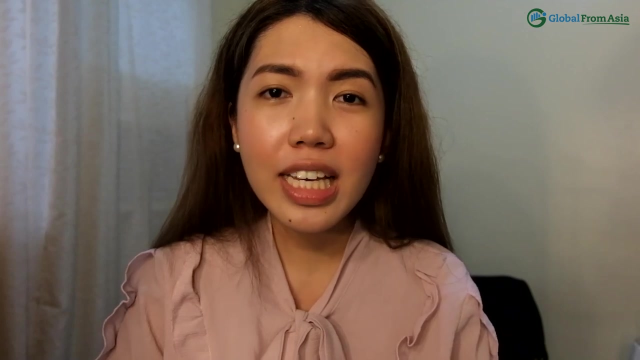 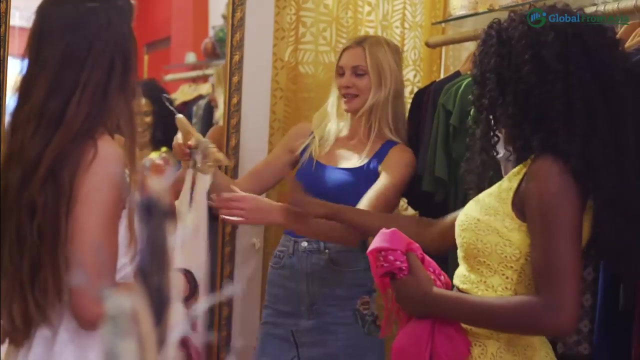 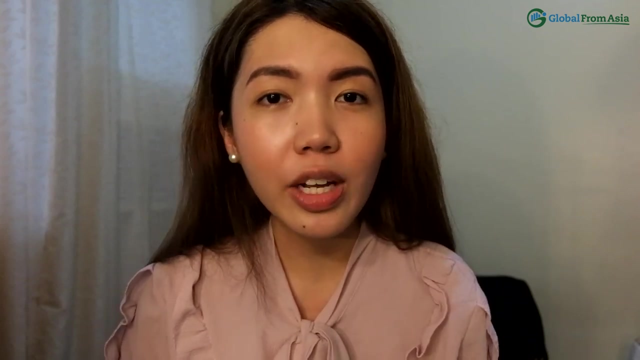 So everything that has to be decided on, the elders would be the ones to decide whatever step to do. So this is contrary to the practices in the West where each individual can decide for their own. So it is also evident in the Eastern world that the children would take care of their parents when they grow old. 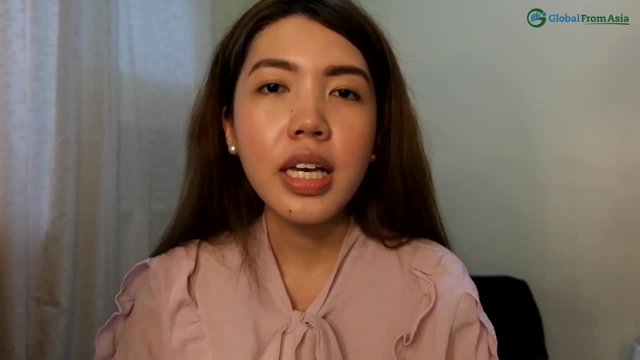 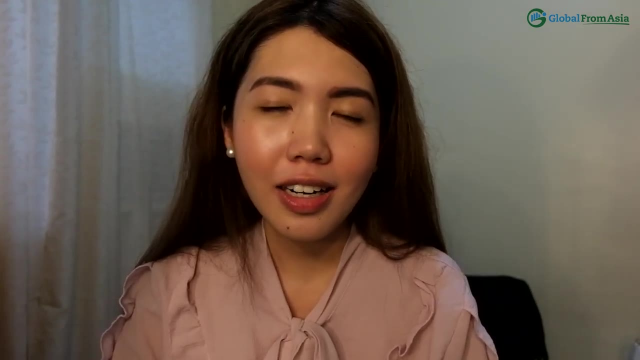 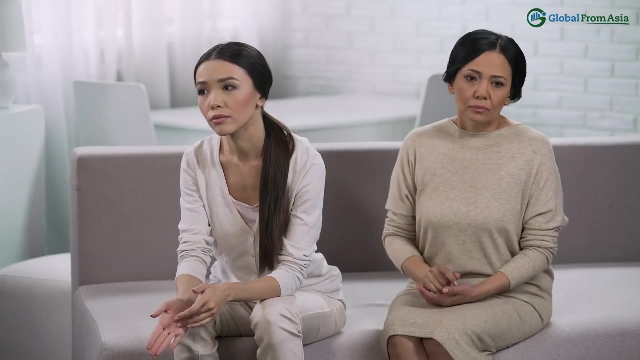 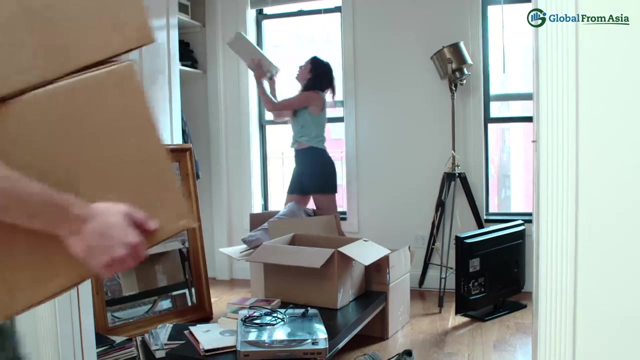 However, this is not common in the Western world. Lastly, when it comes to marriage, the arranged marriages are actually common in the Eastern world. They believe that love comes after marriage. However, this is not the case in the West. However, this is different in the West, where they believe that love comes before marriage. 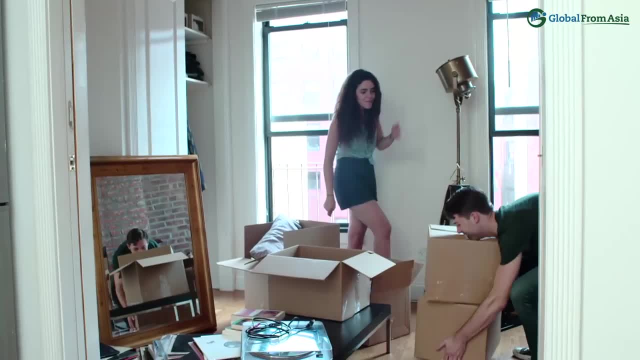 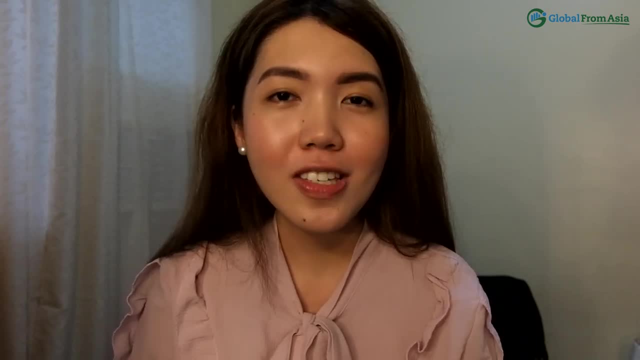 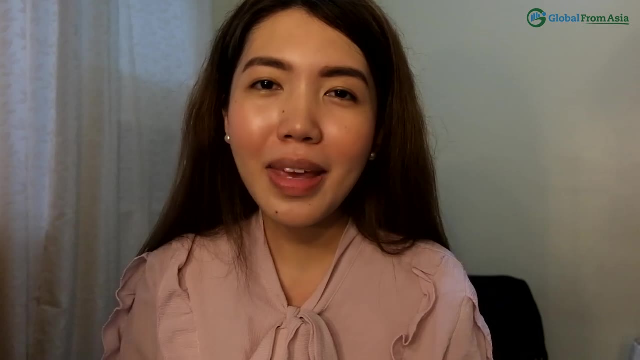 So they don't actually practice arranged marriages. So for the Easterners the arranged marriages are done by the parents or the elders in the community or in the family. So that is what makes these cultures different from each other. See how these cultures vary. 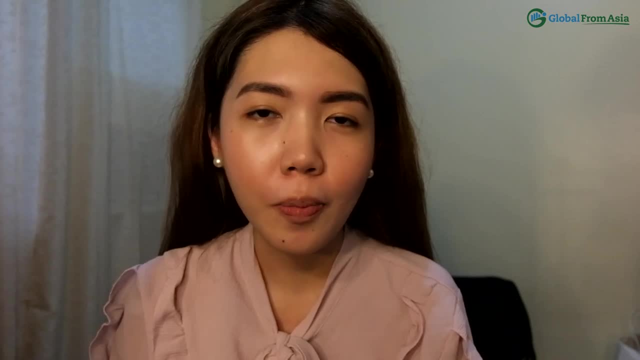 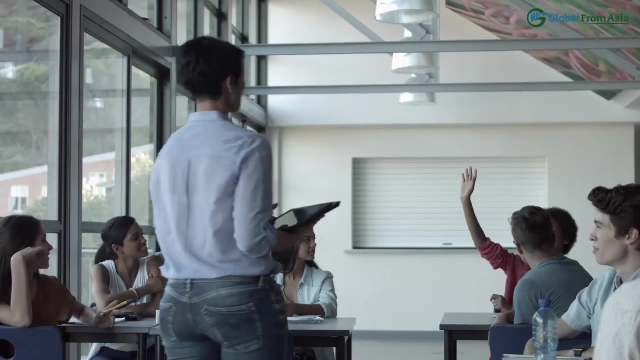 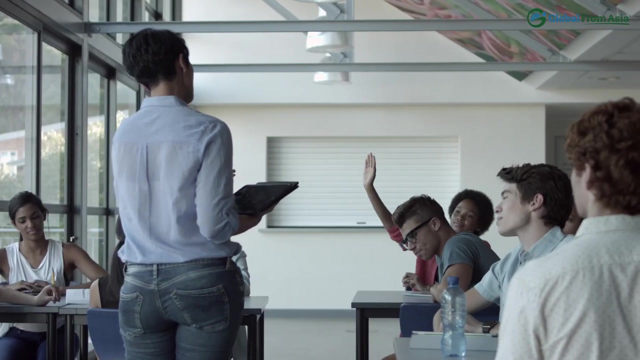 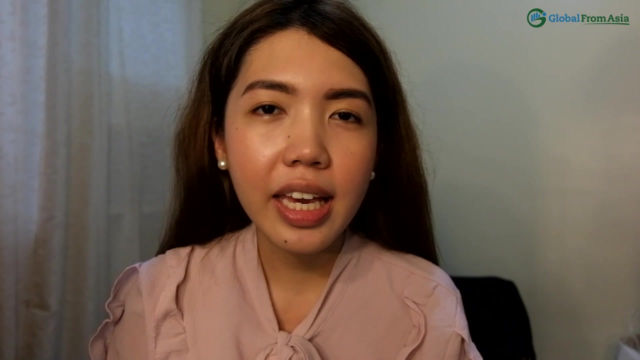 Now let's proceed to the education systems. between the two, Number one creativity versus hard work. So for the Westerners, they value more on creativity, So they have different styles that would apply to each individual. And then for the Easterners, they are more rigid in terms of their education. 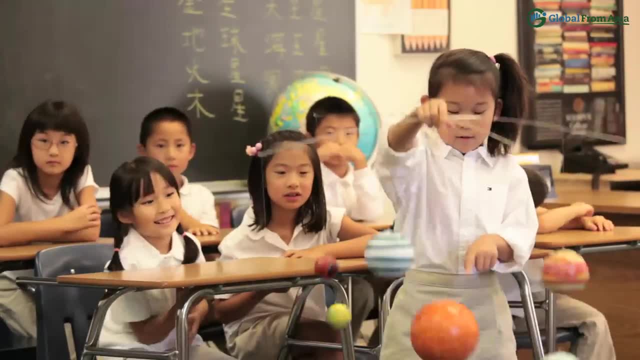 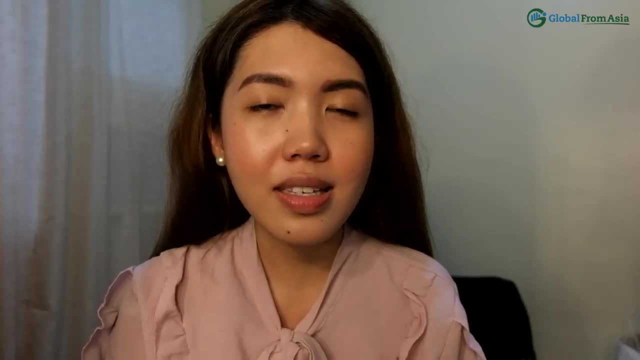 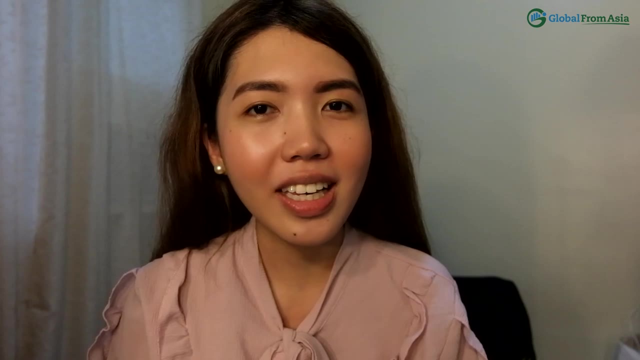 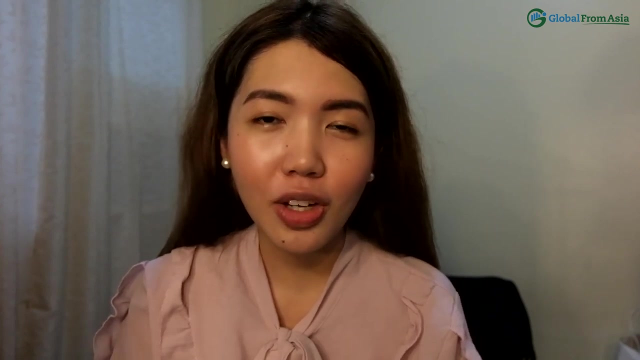 So it actually gives more value to hard work. So they say that nothing is really difficult when you practice so hard, And because of this the Asians or the Easterners actually become more profitable. Second, we have participation versus reception, So the Westerners are more inclined to 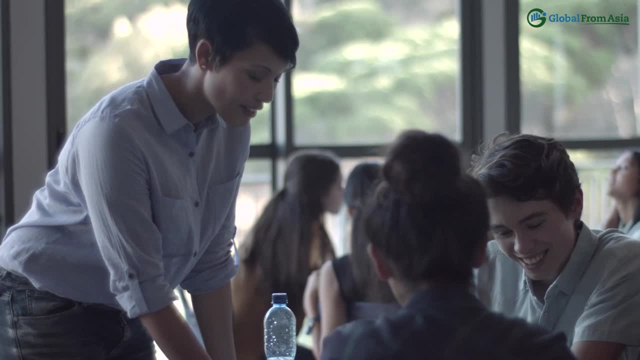 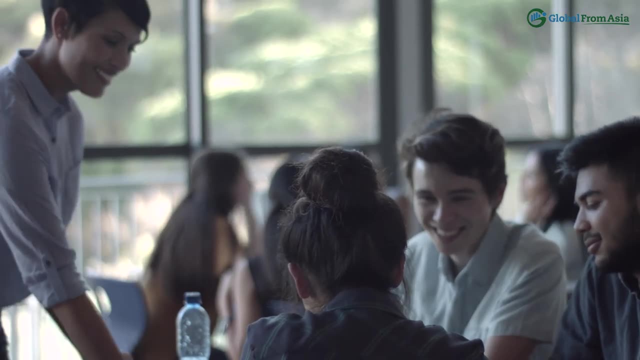 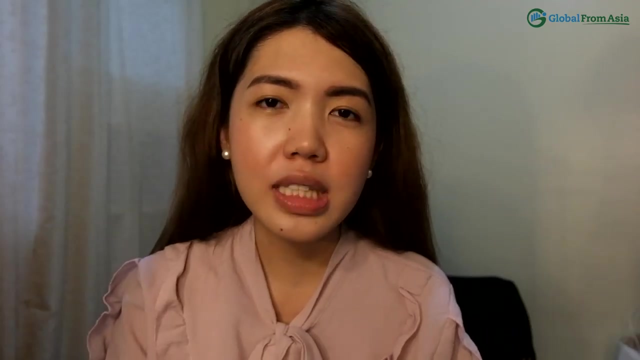 have their students participate in the discussion. They want their students to think critically so they are more open to any ideas that would come from the student. So it's not just a teacher-student kind of flow where the teacher would just say the topics and then discuss about it. 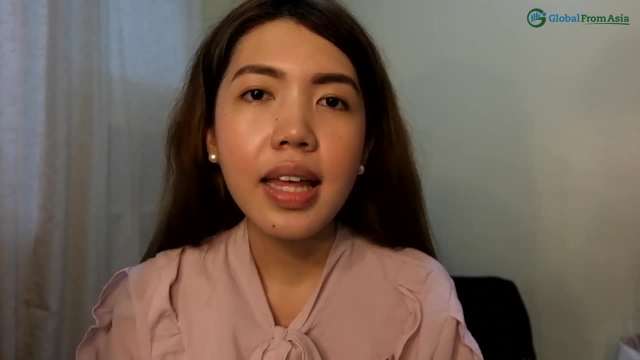 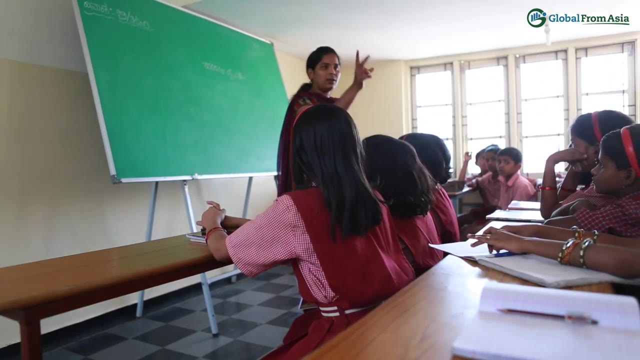 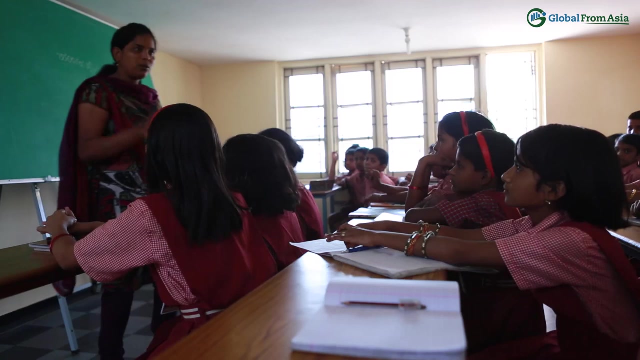 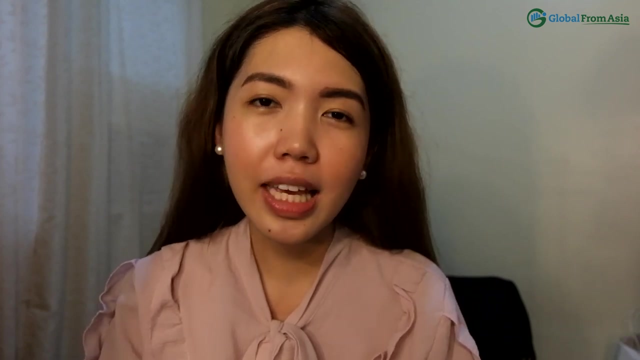 And, unlike the ones in the East, they actually have this reception kind of a learning where the students are more likely to act as receivers of information. It's not too interactive, unlike the ones in the West. okay, So, lastly, in terms of special needs, they have inclusion versus isolation. 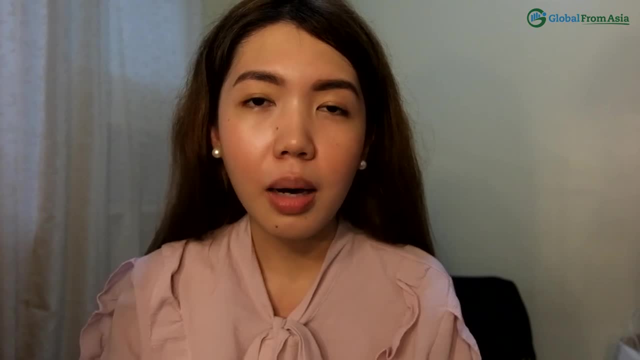 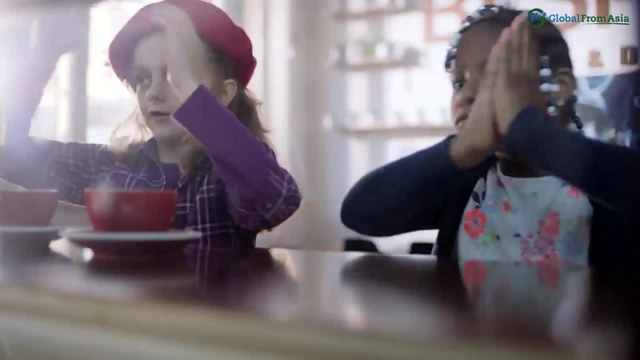 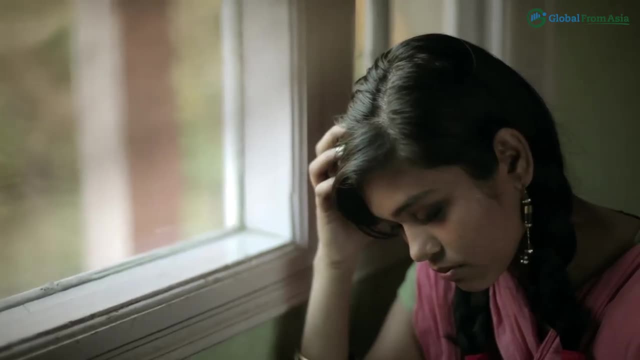 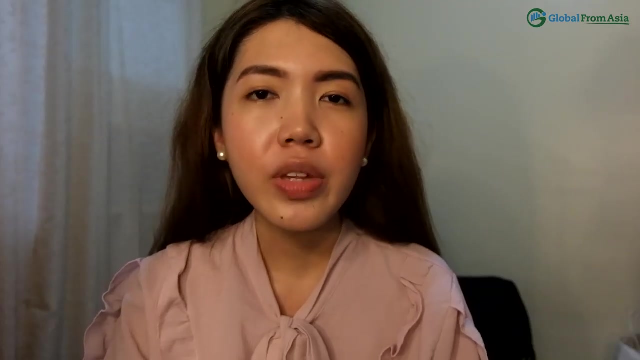 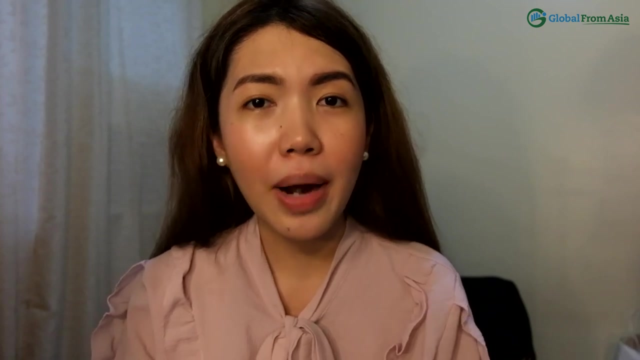 So the child is actually still included in the normal class. So, unlike in the East, the child is isolated, meaning there is a different class for that special child or for that child who needs special attention. So they see this as something that is unbiased but is only practical. 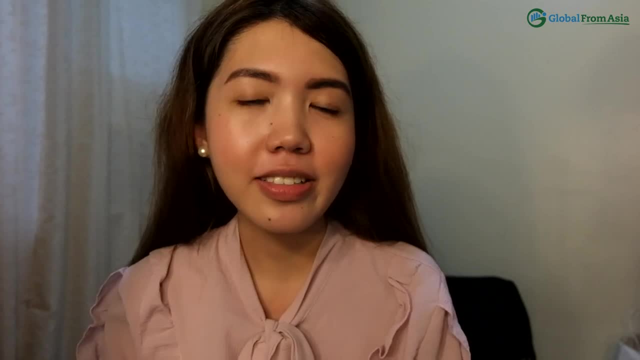 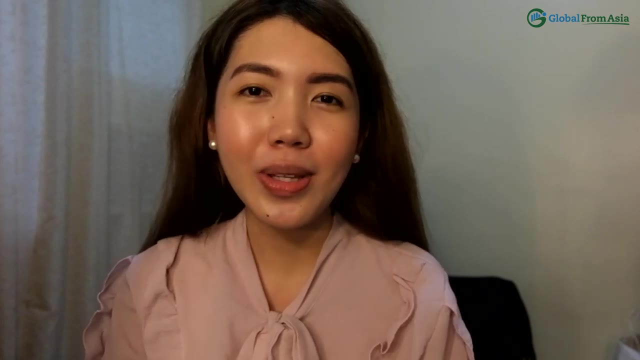 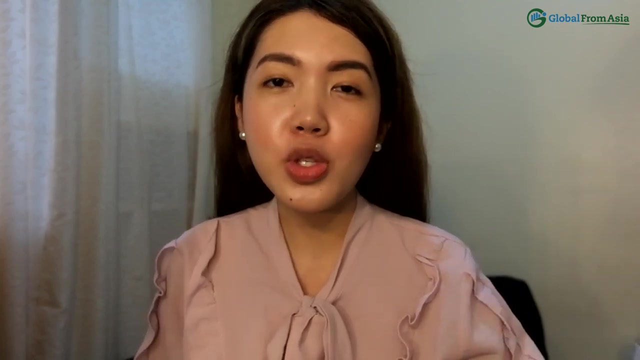 So they think it works best for the child. So that's it. I hope you learned from this episode. So this is how the East and the West differ from each other when it comes to education and culture. So actually we really cannot compare these two. 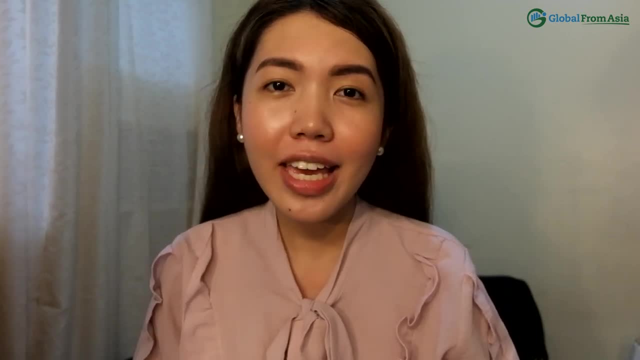 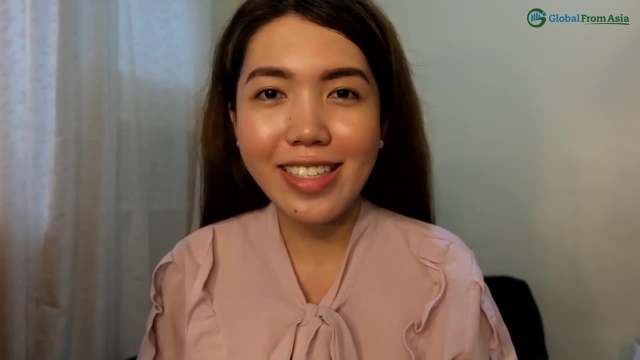 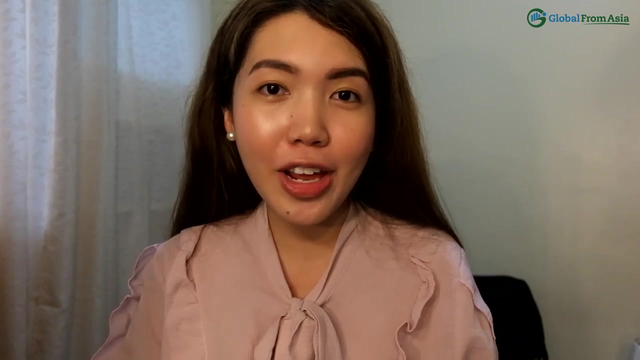 Both are unique in their own ways. However, it is our responsibility to adapt to these cultures, since we already know that the East and the West differ from each other in terms of cultural differences. Now it is your turn. What do you think of the differences between the East and the West in terms of culture and education? 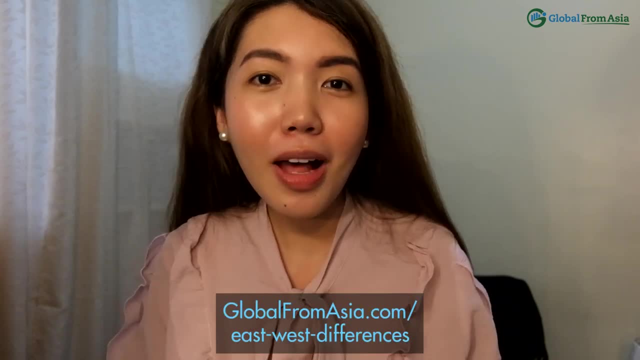 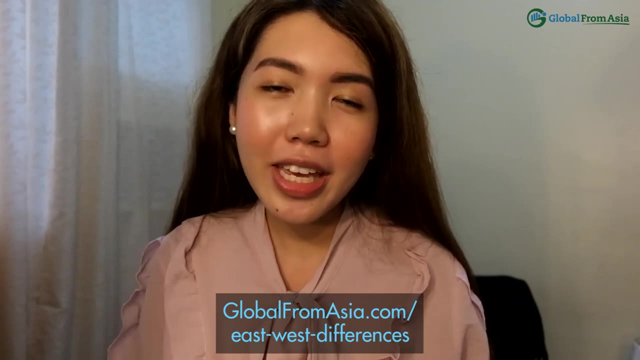 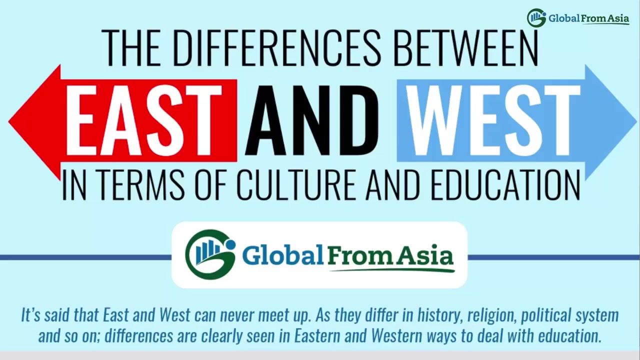 Which one is your favorite. So in the blog post below, you will see a blog section there where you can cast your vote, And also you can read about the other hot trends from our other readers, So please check it out. We have a free infographic that our designer, Alan, has written for us. 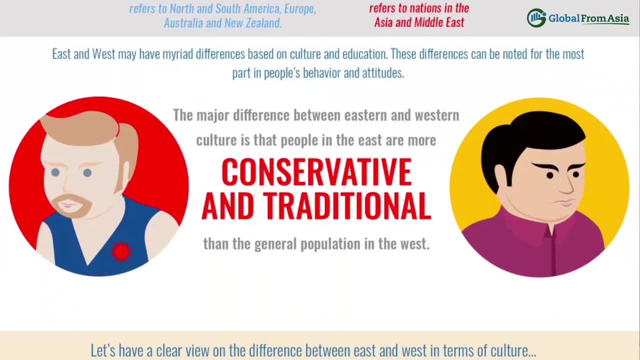 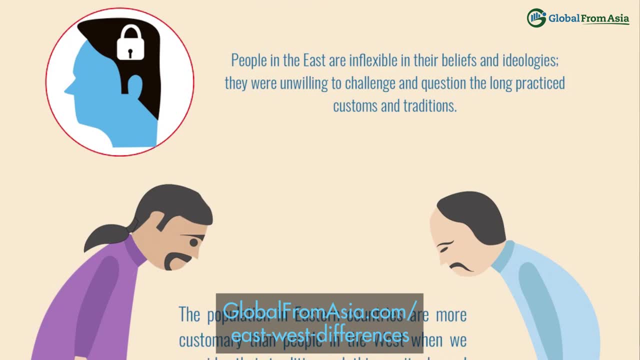 We have a free infographic that our designer, Alan, has written for us. We have a free infographic that our designer, Alan, has written for us. Can you believe it's actually free? So just check it from the blog post below And you can download it and even share it with your friends. 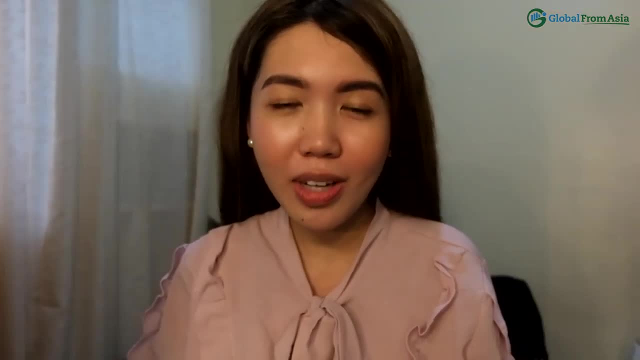 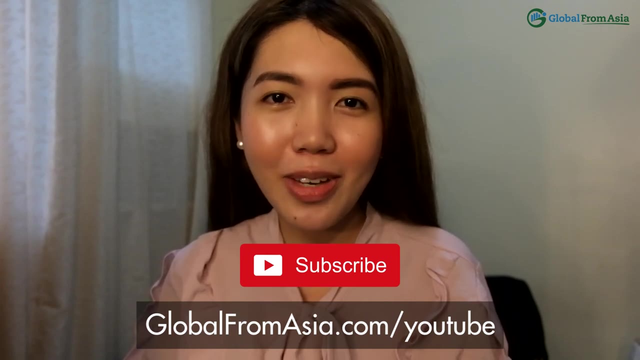 So check it out. And, of course, please do not forget to hit the subscribe button below. Thank you so much for watching. This has been Laika, and I will see you in the next videos. Bye, Thank you so much for watching. 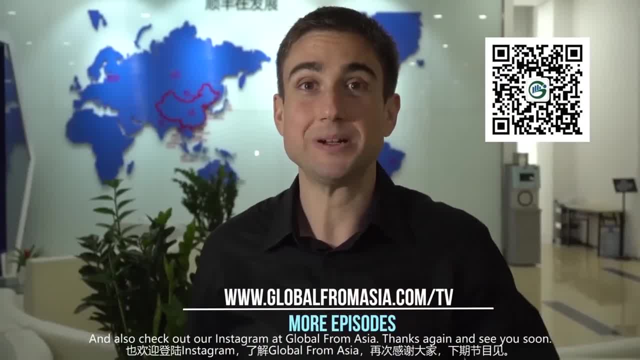